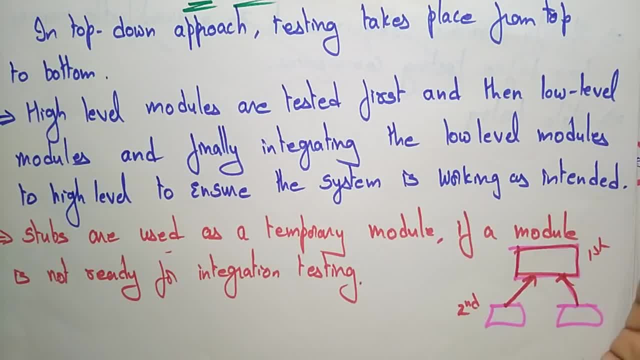 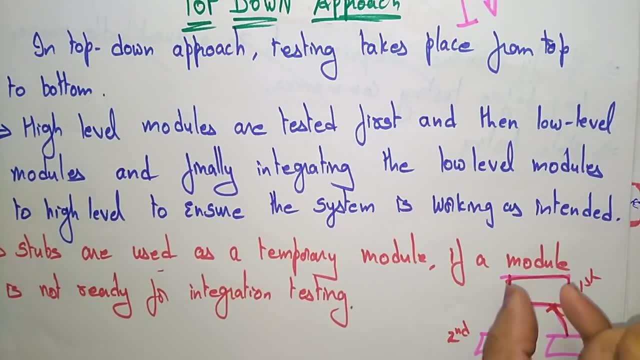 make the system is working. So this condition, this way of testing, you call it as a high level module experiment. Then you also use the top down approach. So what I had done here: I just tested the first module and after that I tested the low level modules. 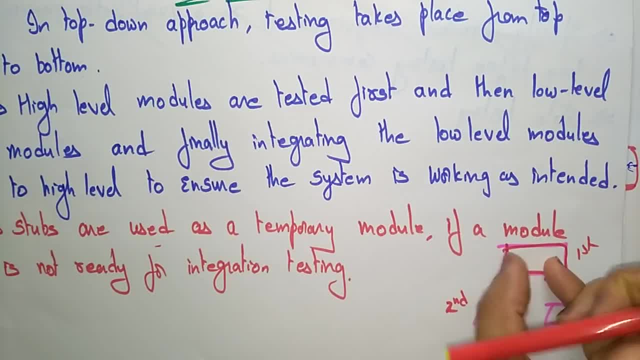 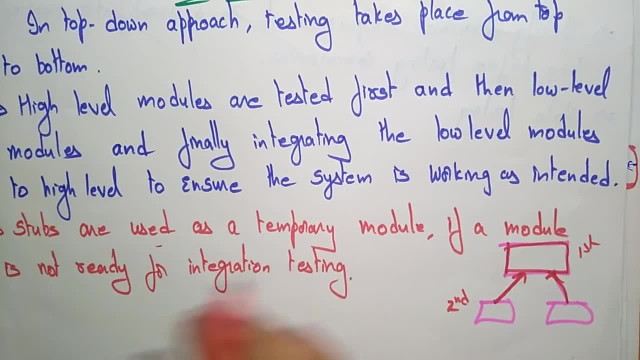 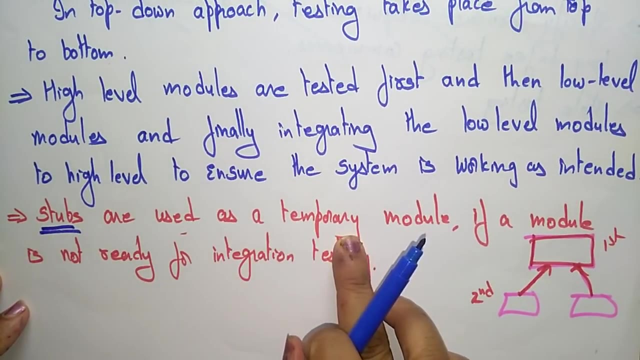 Again I integrated the low level modules to high level module and again I tested. So before dividing I test. After dividing also I test. So here the stub-sor used a concept. Stubs is here Stubs warrior, used as a temporary module if the module is not ready. Devil另外i wçël. 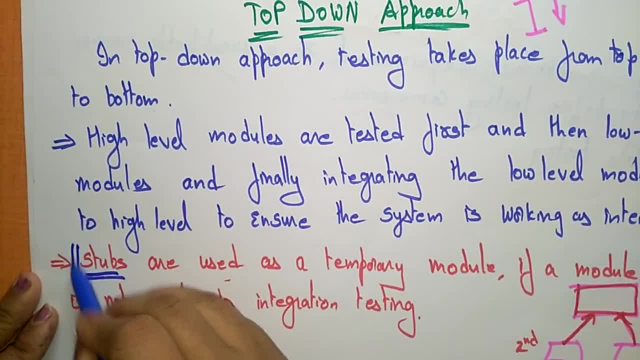 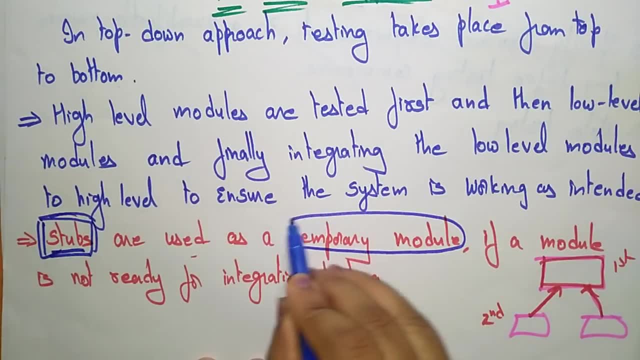 12 for integration, again top down approach. So what I had done here, I just tested the first module And testing. So in the top-down approach we use the concept stubs. So what is a stub? A stub is nothing but a temporary module. The one thing you have to be note that stubs are a dummy. 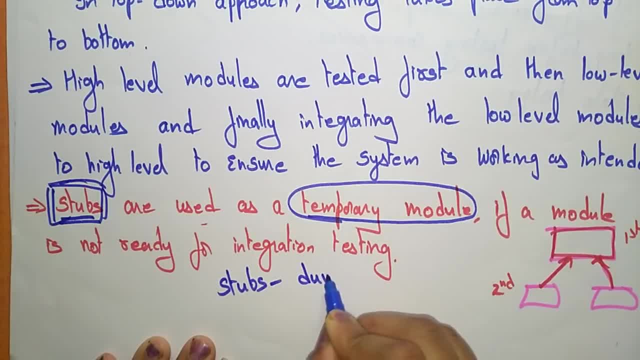 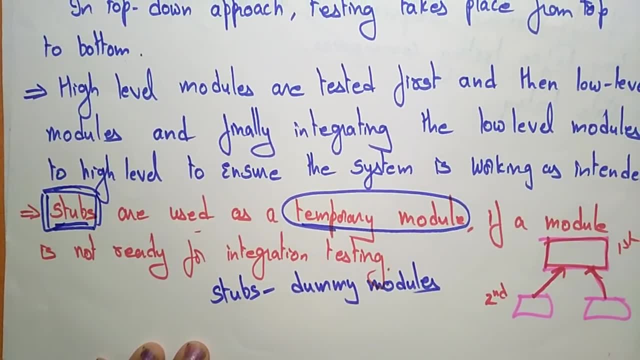 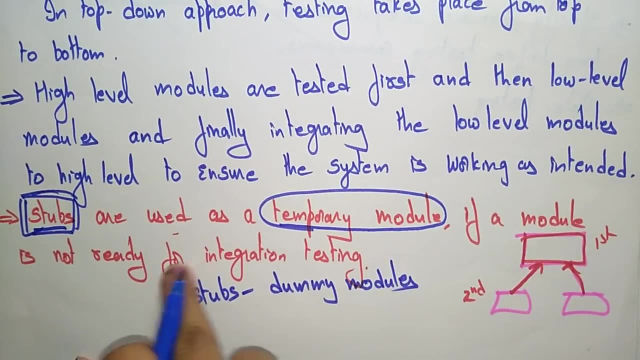 stubs or dummy modules. It's just a dummy modules, It doesn't have anything. okay, only for the sake of reference. only you are keeping the dummy modules. So stubs are used as a temporary modules If a module is not ready for integration testing. suppose this is one, the main page and here this: 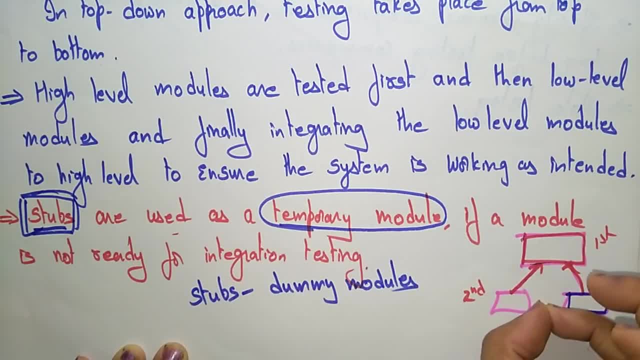 module is still not ready. but if you want to done an integration testing on this too, but this module is not ready, you'd keep. instead of this module you can put stub here. That is a temporary module. So if integration is not ready, if it is not ready for integration test, if this module is. 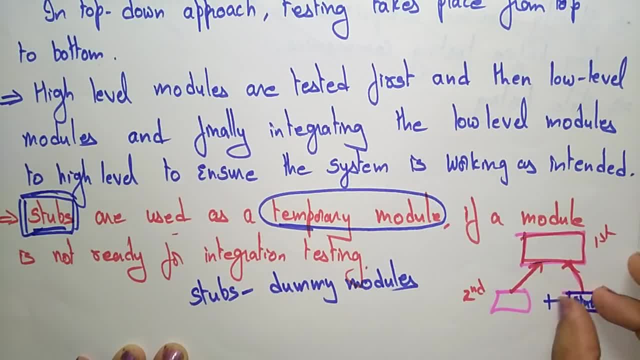 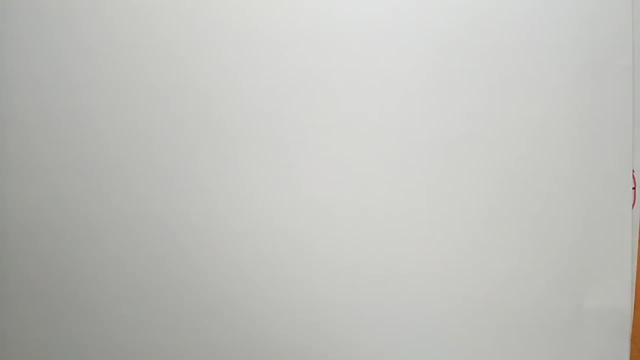 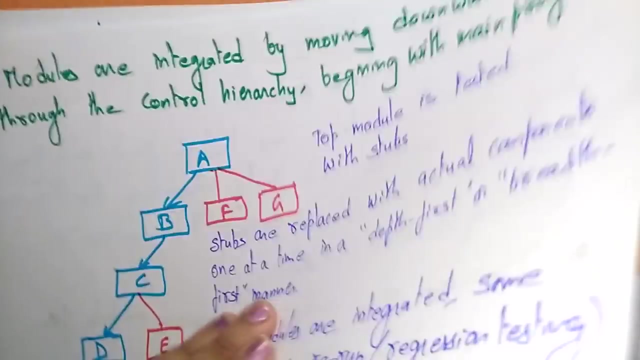 not ready for integration test, then you can make one stub here and you perform integration testing here for the final thing. so this is about it, a stub. so the stubs is always used in the top down approach only. so let me explain about that stubs here. so here is- i'm taking one example- that 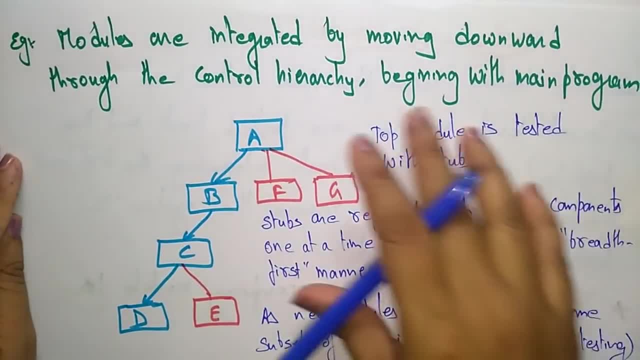 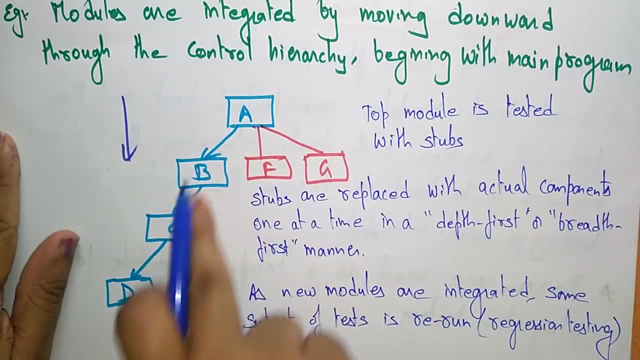 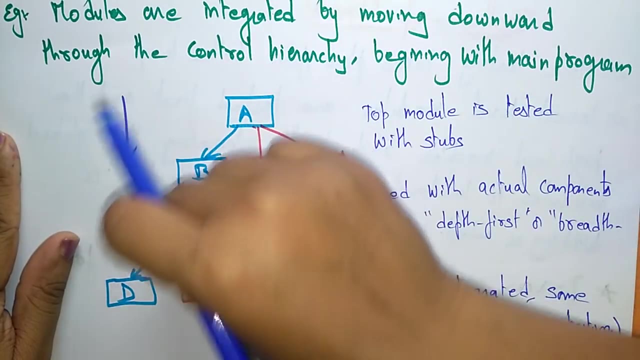 is, the modules are integrated by moving downwards. so this is a top down approach. so the modules are integrated by moving downwards through the control hierarchy. one hierarchy is following, beginning with main program. so this is a main program that i have divided into a, b, c, d, sub modules. okay, so 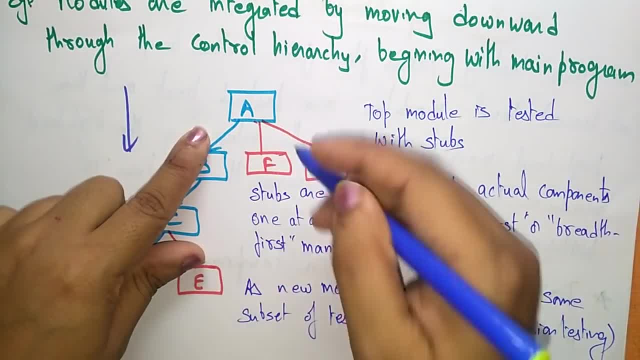 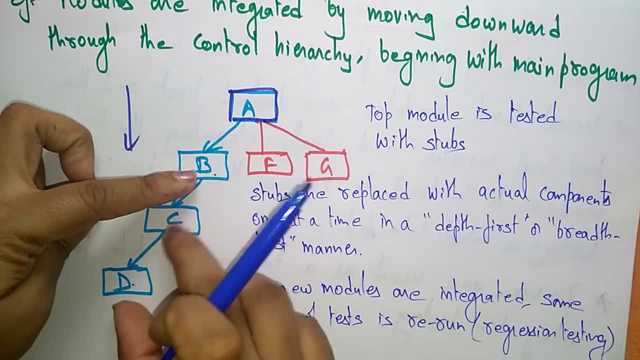 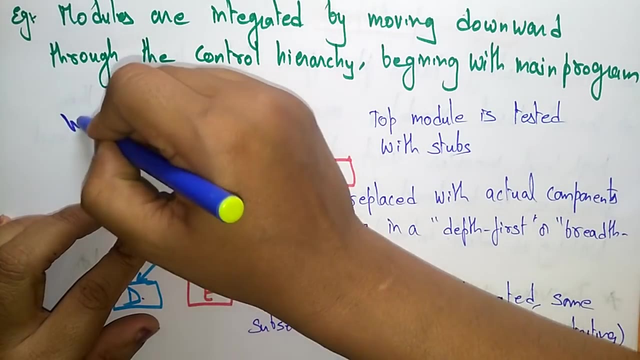 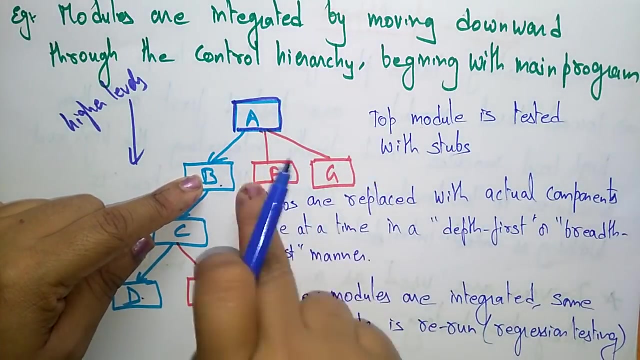 the top module is tested with stubs. so how can i test this a module here? b is there, but cd is not ready. the cd is not ready. so first, in the top down approach or in whatever it may be, first you have to test the higher levels. if you want to do that, test the higher levels. the b is ready, but cd is. 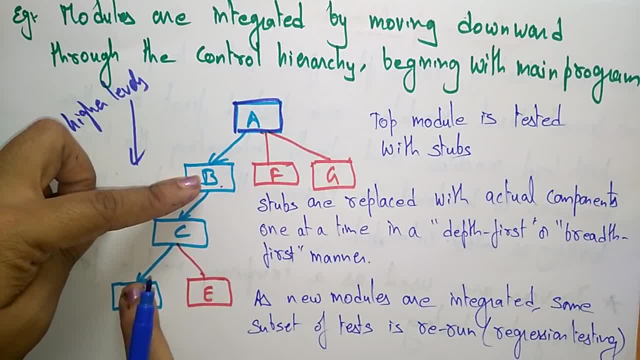 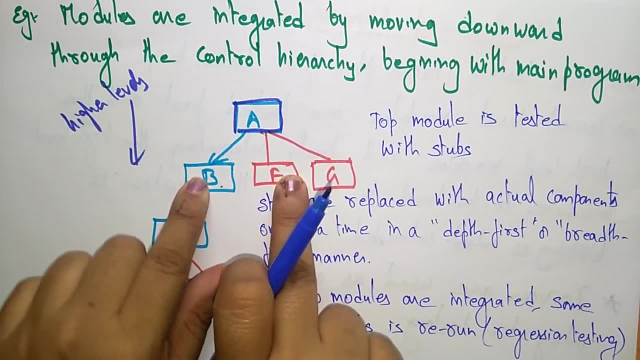 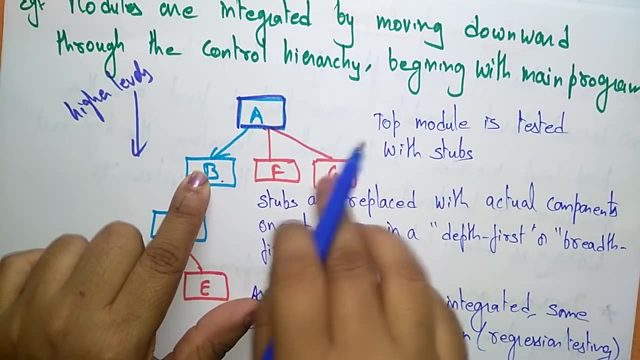 not ready because they are still in, has to perform unit testing. okay, they are not ready, they are doing unit unit testing. so you just keep some dummy modules. that is fg. the top modules are tested with stubs. here fg or stubs. after that the stubs are replaced with actual components. 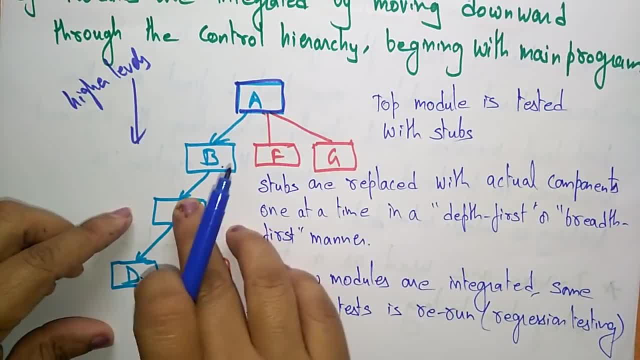 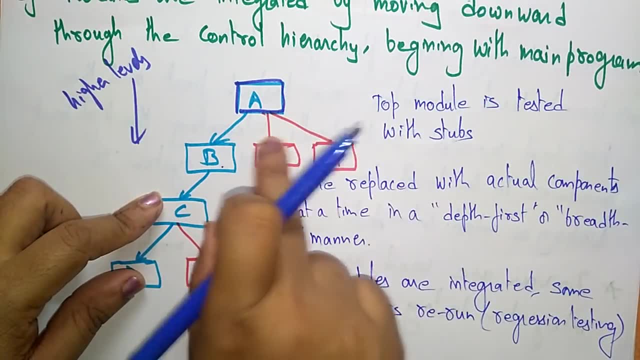 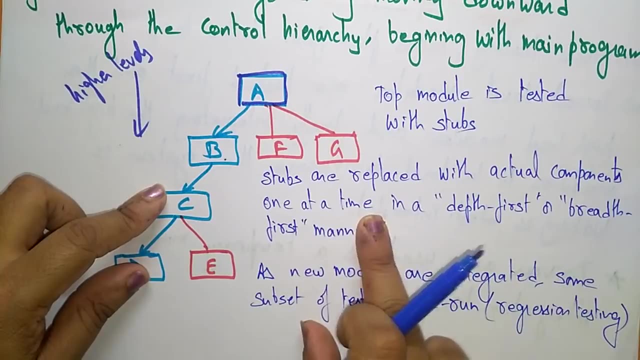 one at a time. so here. so after completion of this cd, unit testing is over. if these modules are ready for integration, then they are replaced here in the place of fg, they are replaced. okay, so the uh stubs are replaced with actual param components, one at a time, by using depth first search or. 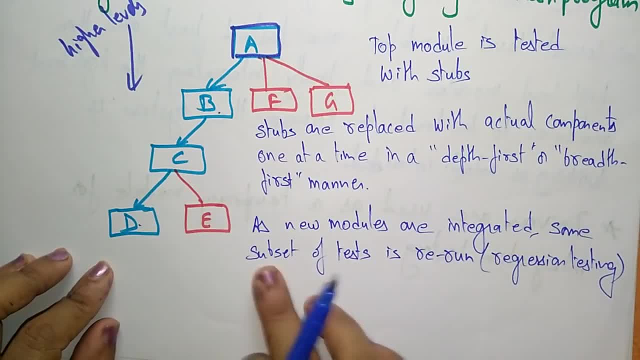 breadth first search manner as new modules are integrated in the top direction. sub modules are self-proclaimed and they are replaced by other components, one at a time are followingona. the top modules are some subset of test is rerun. that will be telling the regression testing. it is one of the regression. 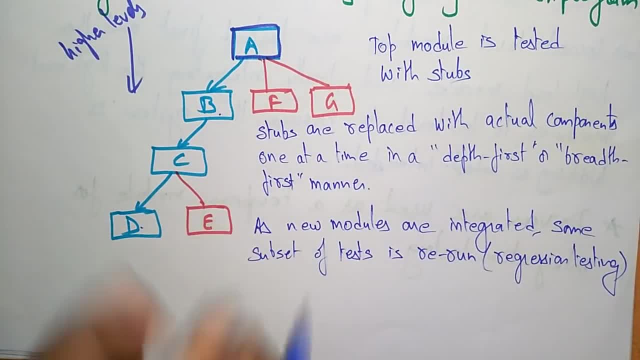 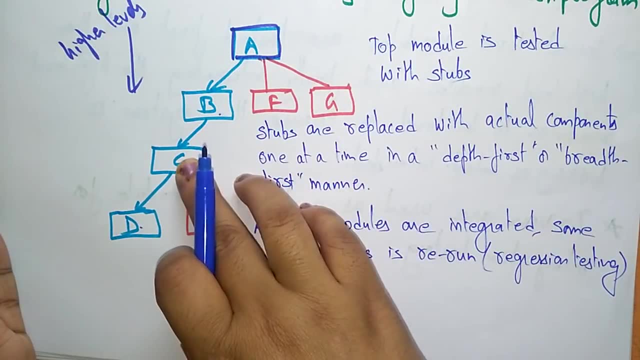 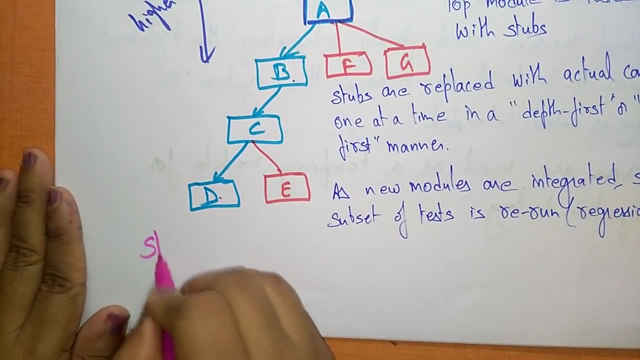 testing methodology. so this is what exactly the testing will be done. this is following the top down approach from top. you are checking everything, okay, so let me take another example to explain about this: stubs here. so i said stubs are used for in, only in top down approach, in the top down. 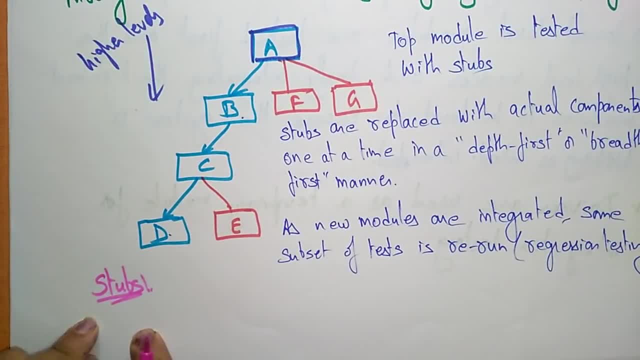 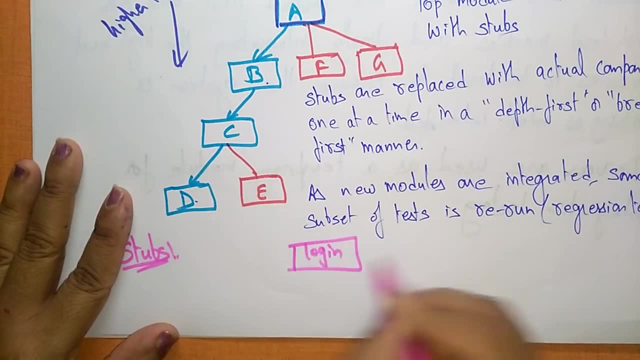 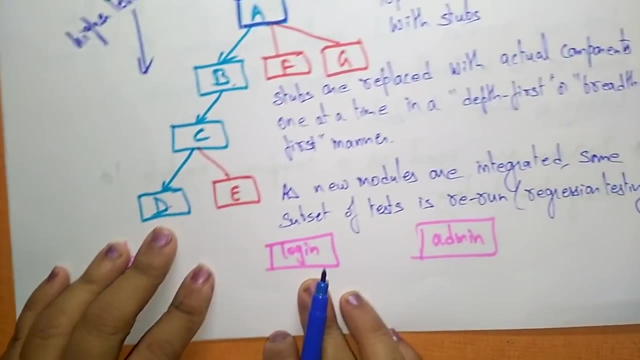 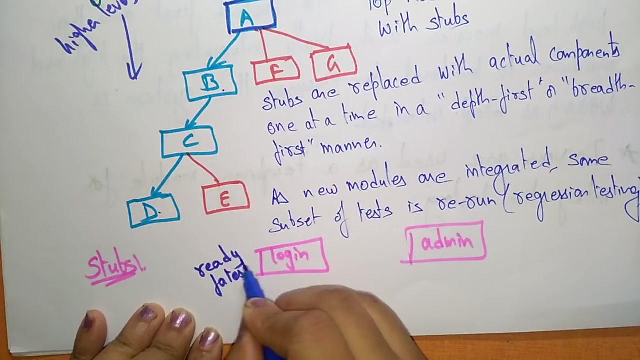 approach. we use the concept stubs. the stub is nothing, but it is a dummy module. okay, so here a login page is there and here an admin page is there. okay, so the login page is ready for testing. so this page is already ready for testing, but admin page is still under development.